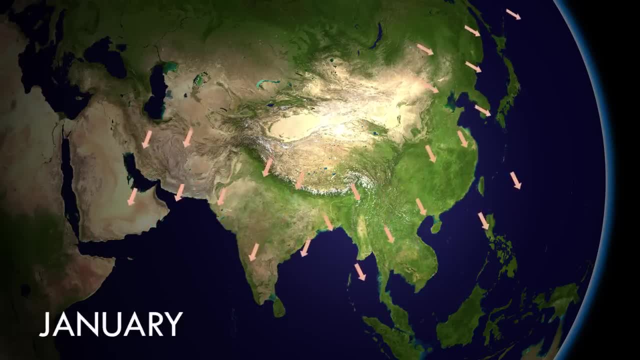 this change in wind direction occurs around the whole of one side of the world's largest continent, producing a wet summer and a dry winter across a huge area of Earth. Now, those of you familiar with tropical climates will know something of wet and dry seasons. 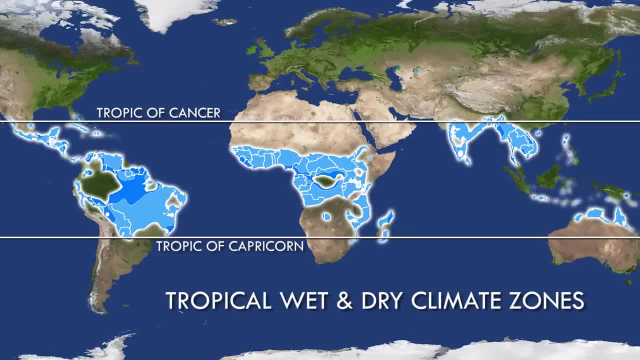 and how the trade winds of the tropics determine these. I covered this concept in my episode on Tropical Wet and Dry Climates in my other series. They always occur within the tropics of Canson, Capricorn, from 23 degrees north to 23 degrees south. 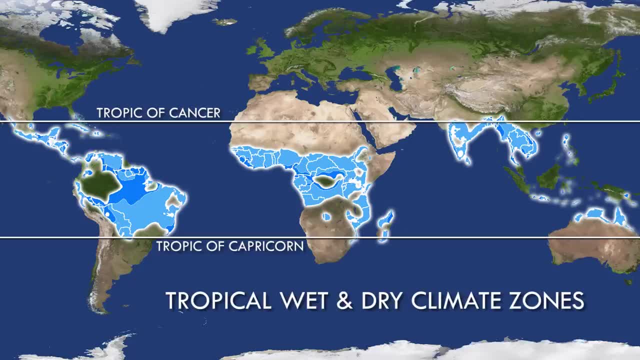 So wet and dry seasons related to changing wind direction are not unique to Asia. So wet and dry seasons related to changing wind direction are not unique to Asia. So wet and dry seasons related to changing wind direction are not unique to Asia. What makes the Asian Monsoon stand out are two things. 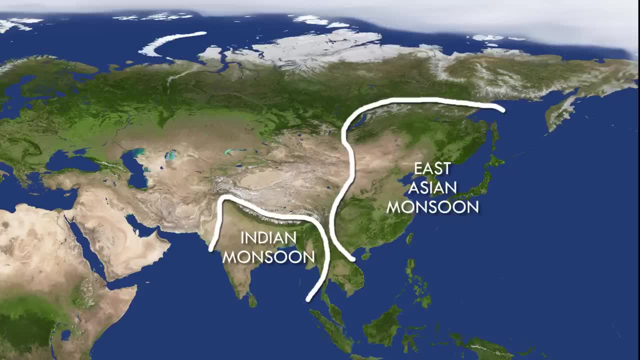 The great intensity of the wet season in the Indian subcontinent and the extension of the wet and dry season pattern in Eastern Asia way beyond the tropics into the temperate continental and subarctic latitudes. So the Asian Monsoon has these two notable aspects. 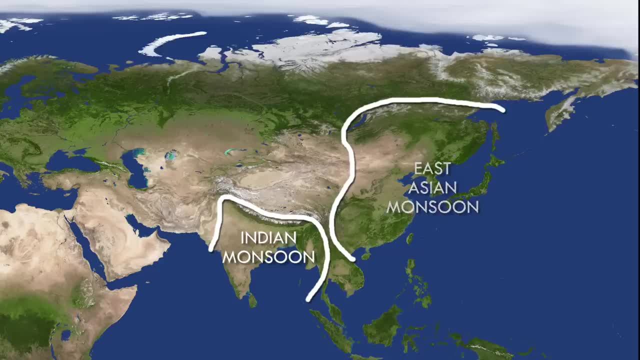 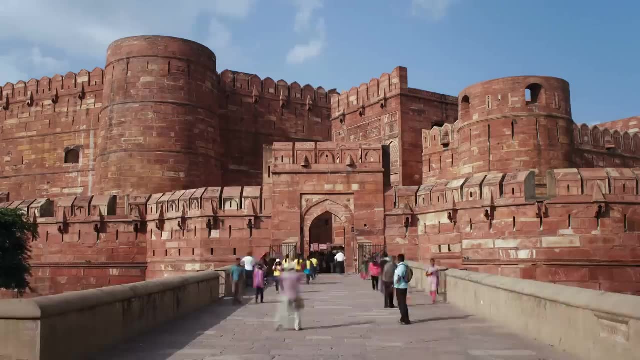 and each defines the two broad halves of the monsoon: The intense monsoon that affects India and Bangladesh. The intense monsoon that affects India and Bangladesh is the most well-known and it determines the lives of the 1.5 billion people that live there. 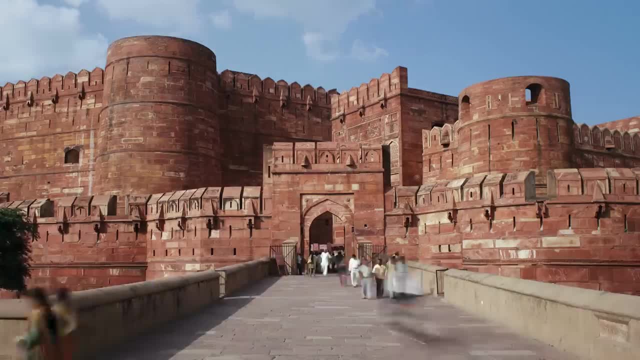 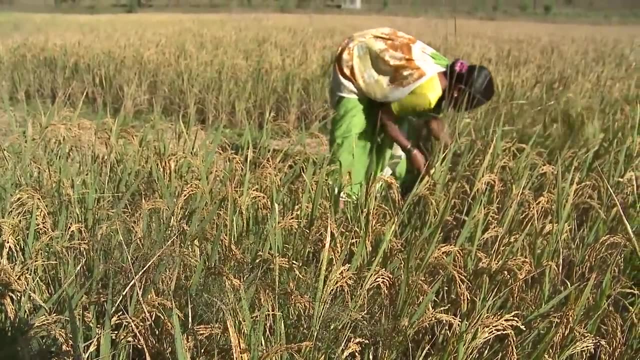 more heavily than any other weather system in the world. The economic fortunes, even the survival itself of these populations depends upon the timing and severity of the wet season that washes over these lands between June and September. Less well-known is the East Asian Monsoon. 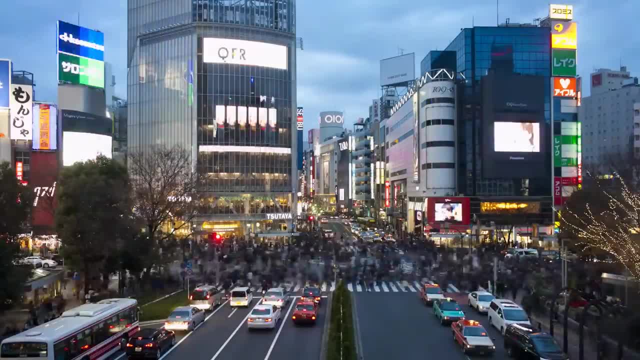 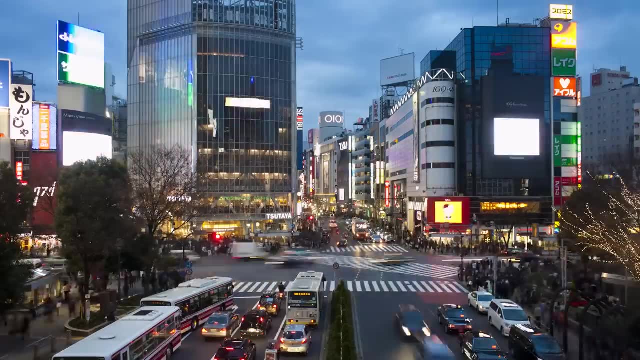 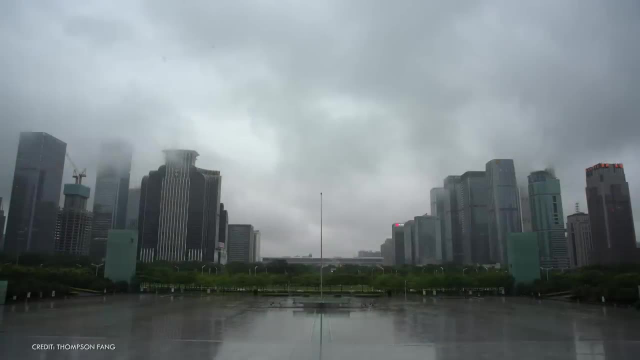 Though less intense, its range is much more extensive and, as many people experience its annual rhythm, with Eastern Russia, among others, and most of China are affected. Before we look at these areas in more detail, we should try to understand what dynamics are special to the Asian Monsoon. 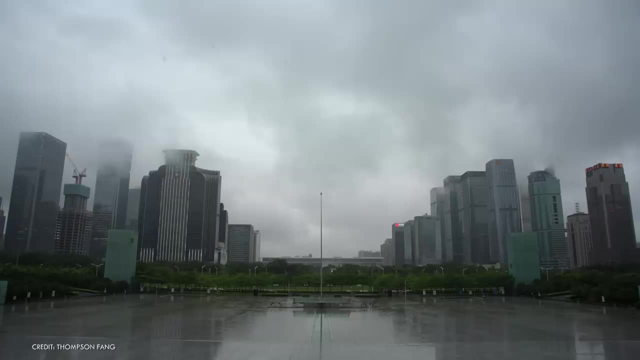 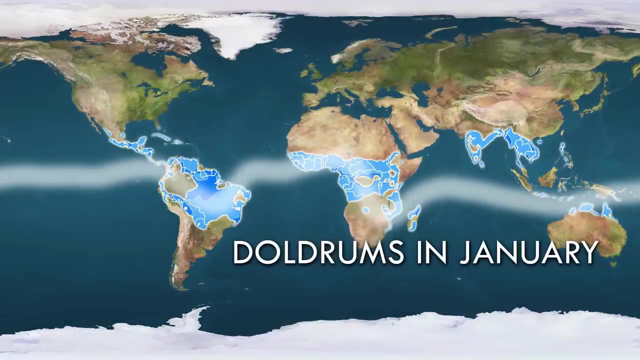 This weather system and its causes are complex and even to this day, are not fully understood. However, it is generally accepted that the two strongest influences are the seasonal march of the doldrums above and below the equator that affects all tropical, wet and dry climates. 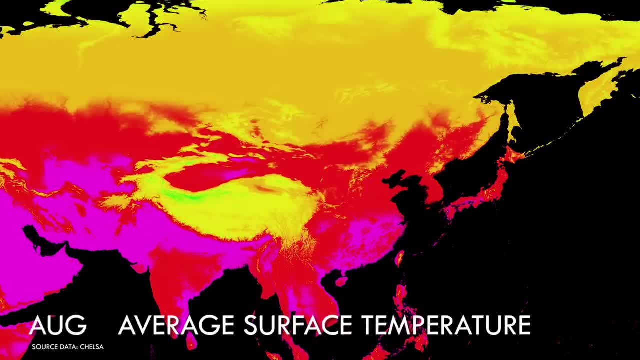 magnified by the seasonal heating and cooling of the climate and the increase in the amount of rain that is caused by the monsoon. and the increase in the amount of rain that is caused by the monsoon. The doldrums, also called the Intertropical Convergence Zone. 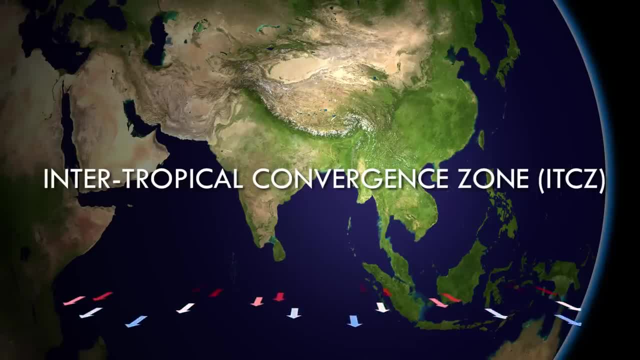 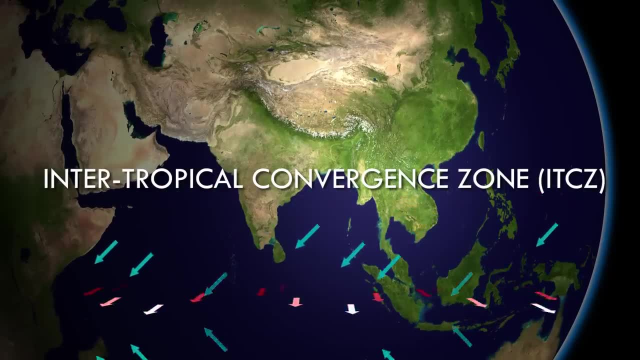 or ITCZ, is the band of low pressure around the tropics where heating from the sun causes upward convection of hot air, leading to a drawing in of air from the surrounding land or sea in the form of trade winds As the global seasons alternate: summer. 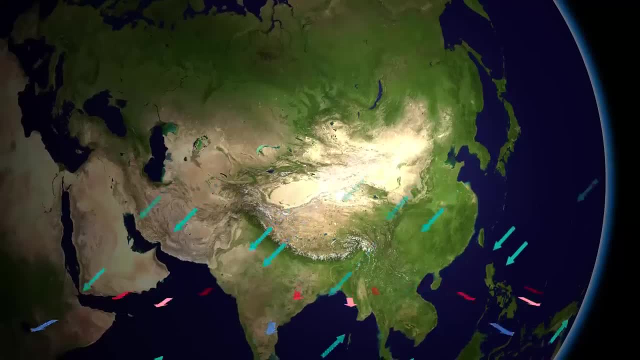 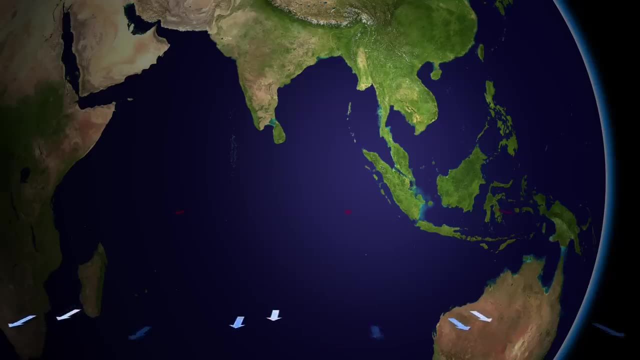 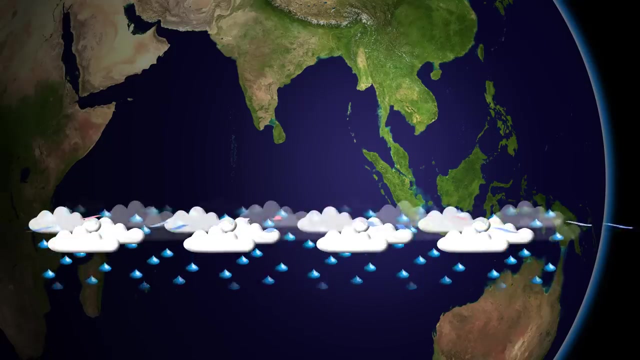 between the northern and southern hemispheres. the ITCZ follows with it, tracking north in the northern summer and then south in the southern summer. This band is almost always accompanied by heavy thunderstorms and consequential rainfall, as the hot and moist air is unstably thrust into the cold upper atmosphere. 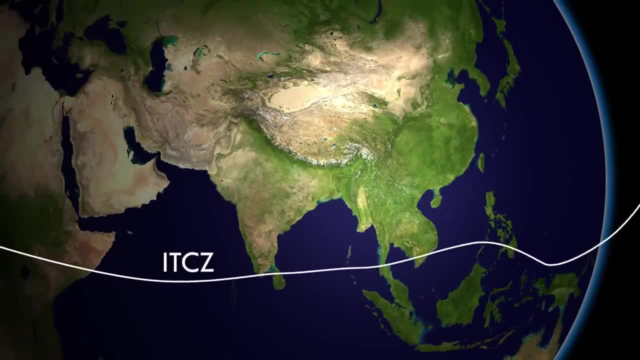 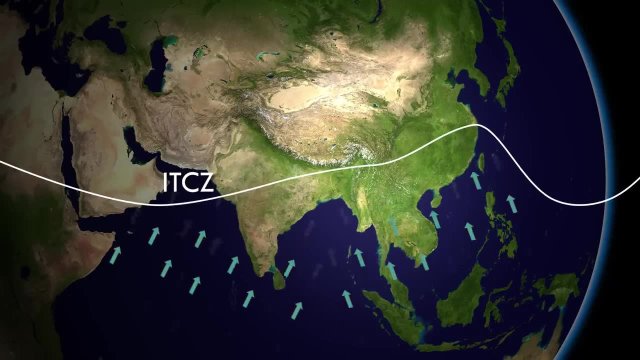 In the northern summer, the ITCZ moves up into India and China, bringing with it southerly trade winds which blow onto the continent from the surrounding seas. This is what brings the rain with the monsoon, as it does with any tropical wet season. 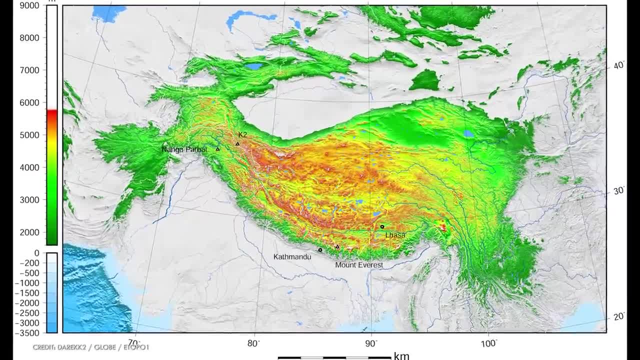 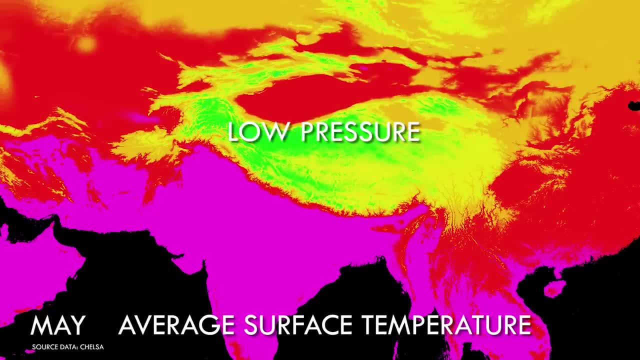 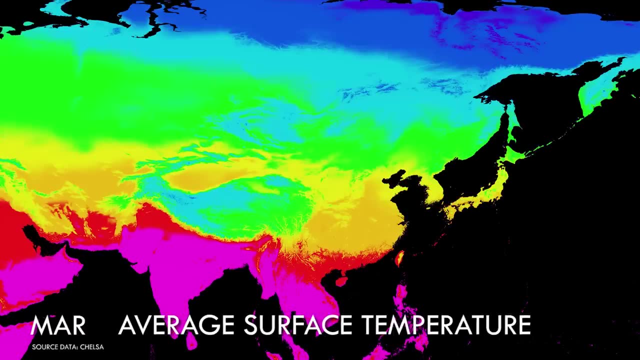 But this effect is strong as it is strengthened further by the presence of the large Tibetan Plateau, the heating of which leads to a deepening of the low pressure, strengthening the monsoon over India far beyond a standard tropical wet season. Additional summer heating of the Central Asian landmass north of Tibet. 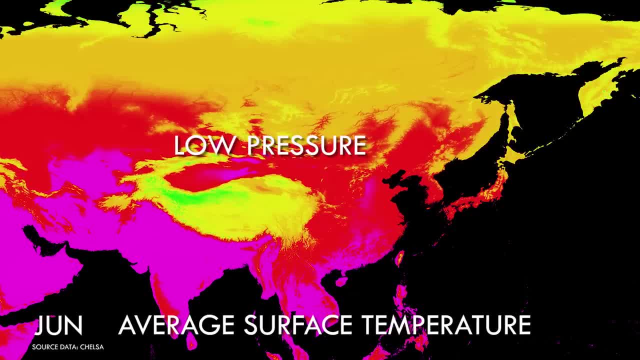 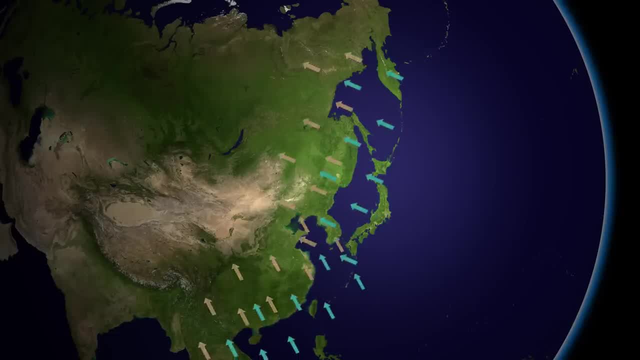 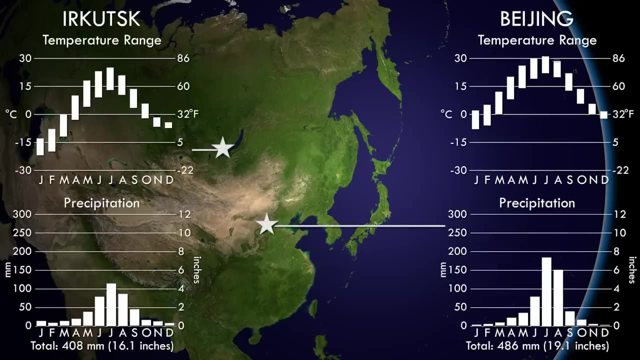 far from the moderating ocean is also strong and extends as far as Siberia, leading to winds blowing in from the Pacific across all of Eastern Asia, from Hong Kong to the Russian Pacific coast. This is the only part of the world where summer peaks in rainfall occur in the mid to high latitudes. 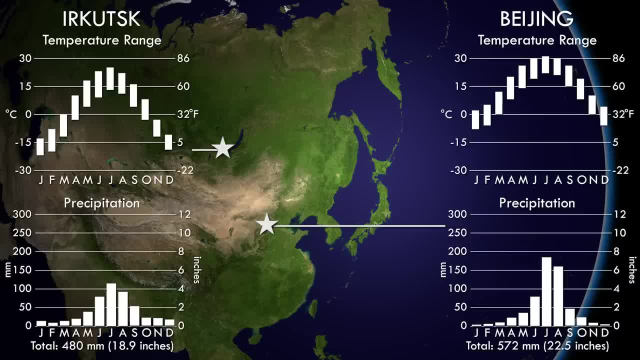 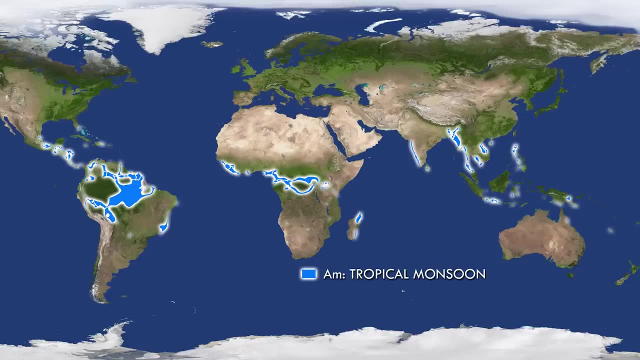 and special climate zones. the continental and sub-arctic monsoon types were designated by Vladimir Kopan to account for this extension into the far north of what is essentially a tropical weather system. While we're on the subject of Kopan, we shouldn't confuse the Kopan climate type AM, the tropical monsoon, with the Asian monsoon. 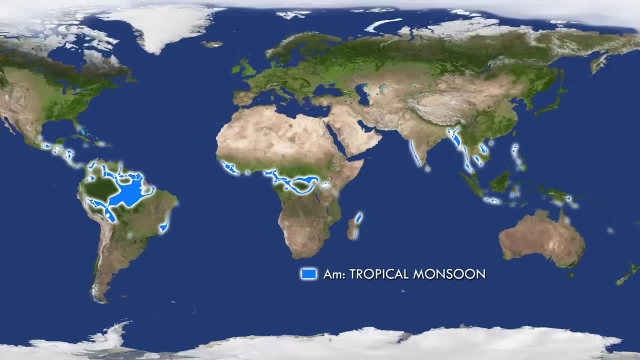 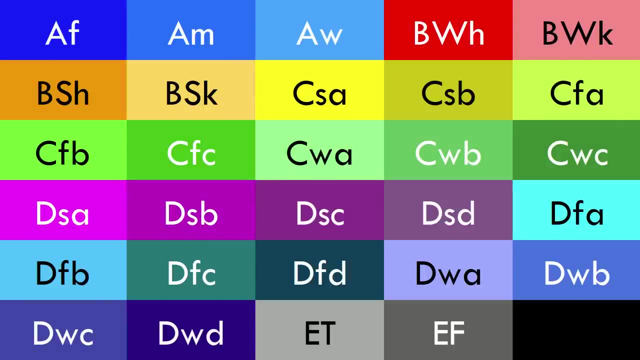 as this zone can occur all the way to the north of India, all over the tropics, from Miami and Rio in the Americas to Central Africa, Indonesia and the Philippines. The Asian monsoon encompasses a multitude of Kopan climate zones, all of which have peak rainfall during the summer. 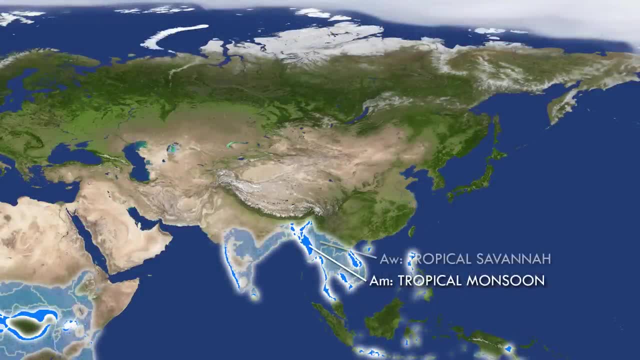 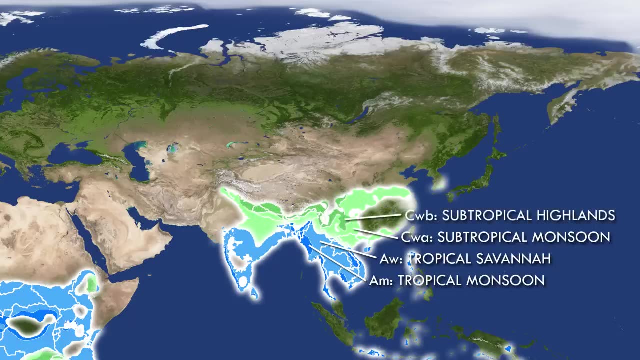 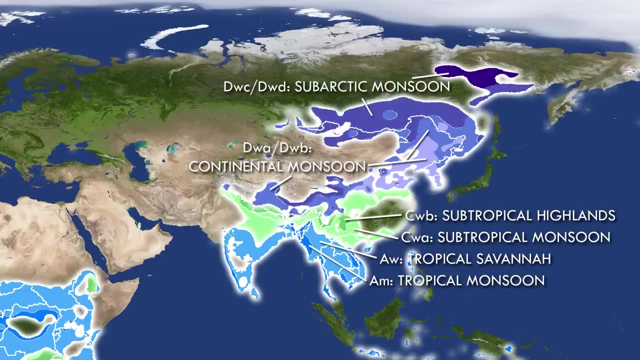 These are: AM- Tropical Monsoon, AW- Tropical Savannah, CWA- Subtropical Monsoon, CWB- Subtropical Highland, DWA and DWB Continental Monsoon. and DWC- Subtropical Highland, DWC, DWD- Subarctic Monsoon. 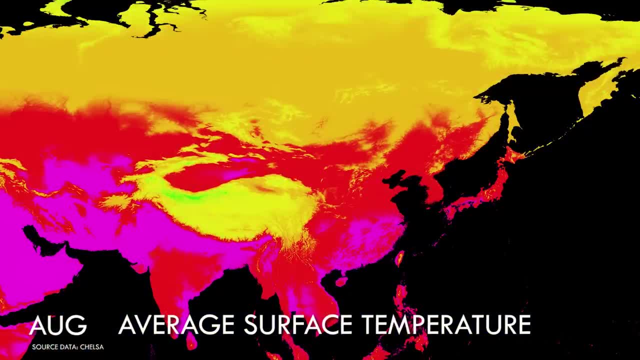 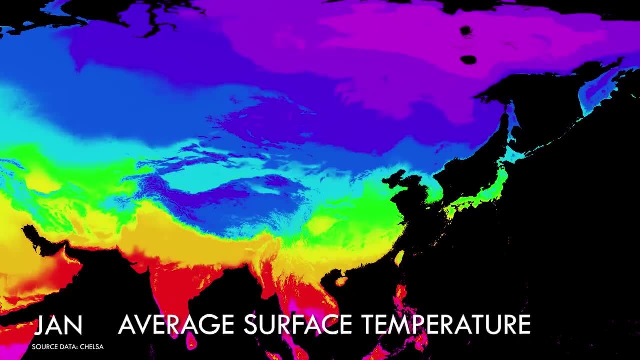 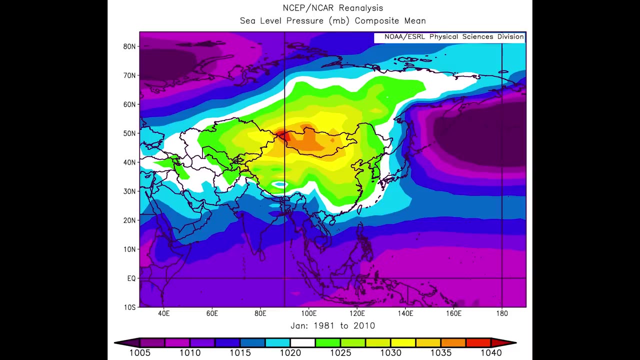 So that's the summer, But what about winter? Well, the opposite occurs. The ITCZ retreats back to below the equator, while temperatures over central Asia plummet below zero, leading to sinking, dense air and high pressure. This high pressure is the strongest on Earth. 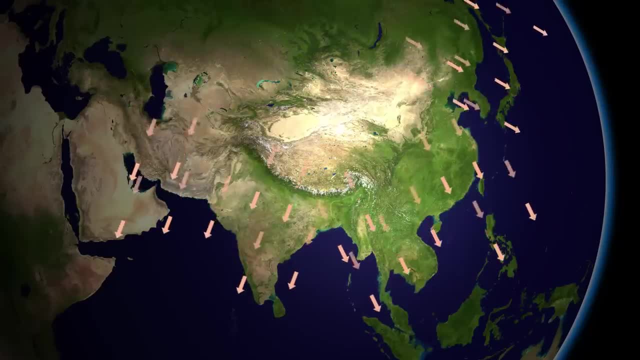 and the continental winds that blow out from it to the oceans lead to dry winters across most of Asia. Only a few of these occur over the summer. few places where such seasonal monsoon winds blow over water in both directions receive rain or snow year round. 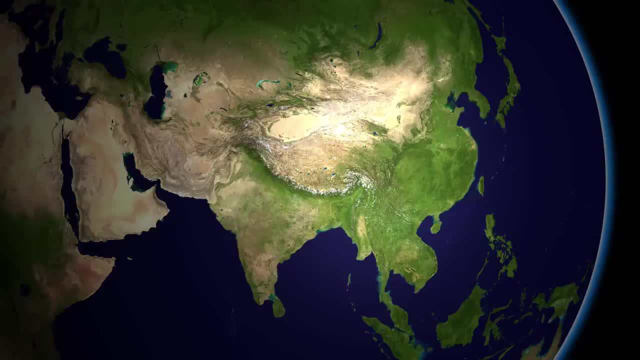 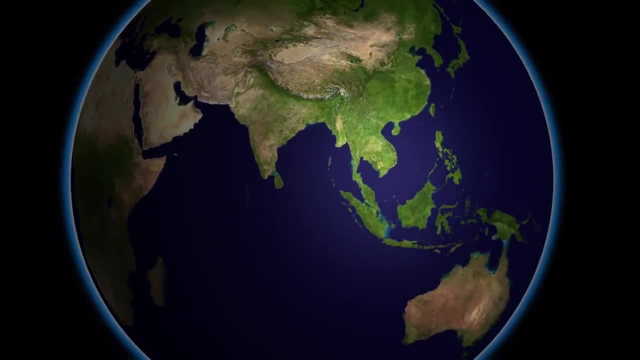 So this, in essence, is the main mechanism driving the Asian monsoon. There is more complexity to it, of course. Australia is believed to have a strong influence on Asia, even though it is a much smaller continent, because it acts as a pressure counterpole with Australian. 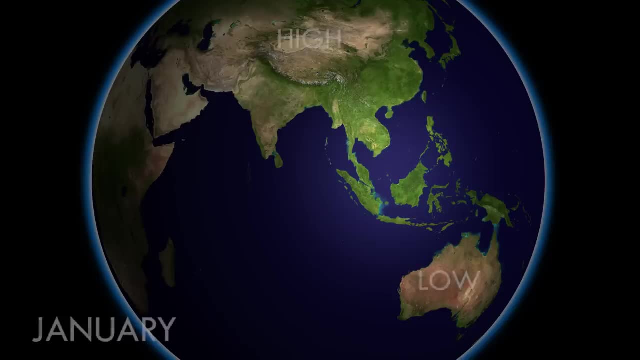 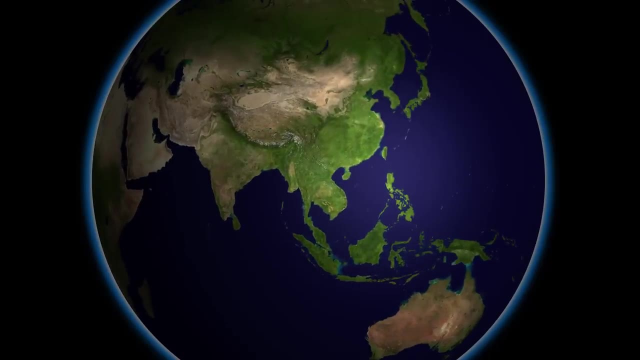 high pressure in the northern summer against the Asian low, and vice versa six months later. The Indian and Western Pacific oceans are the other counterpoles that either provide moist winds in the form of high pressure or sink dry continental winds in the form of low pressure. The monsoon's growth in summer and retreat in winter can be seen in: 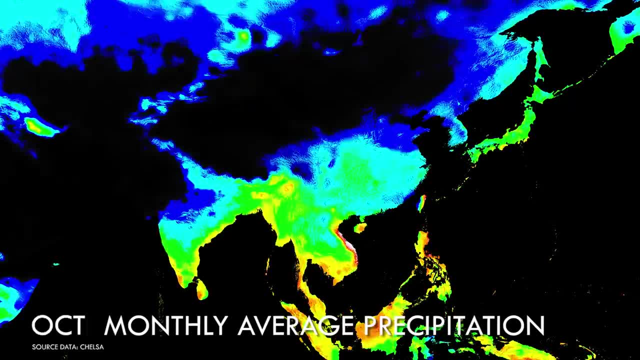 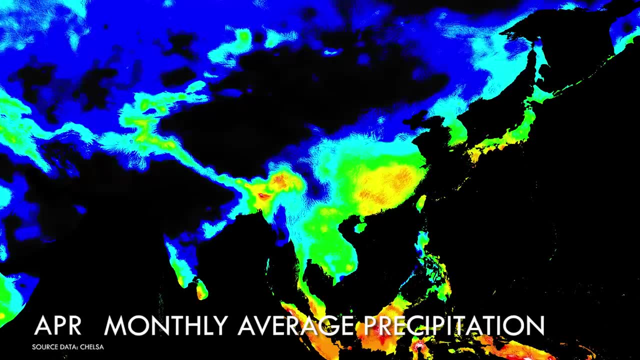 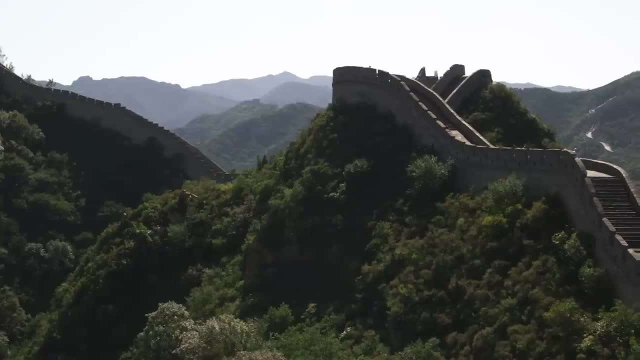 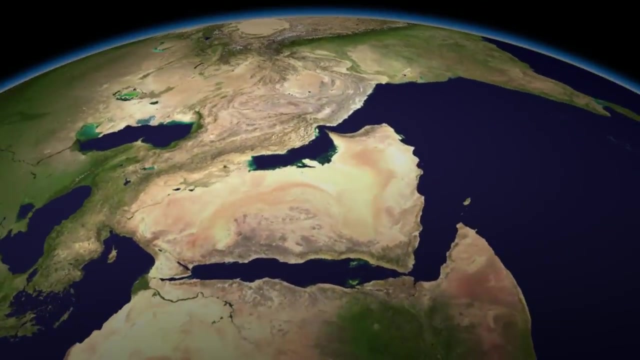 this composite of monthly average rainfall across the continent. It's quite a mesmerising animation, isn't it? I could watch it for hours. Okay, moving on, Let's now journey through the lands affected by the monsoon. The journey starts in the Arabian Peninsula, with the origin of the word itself, but it's also the westernmost point under direct monsoon influence. In summer, winds blow towards the intense low pressure over Central Asia, but because these winds have travelled over the continent of Africa, they bring little to no rain. In winter, the winds switch direction. blowing out from the Central Asian high. This is the best way to get the most out of the monsoon and, once again, a dry continental winds. This is one reason why the Arabian Peninsula is a desert, Moving east into India and the same wind directions south-west in summer, north-east. 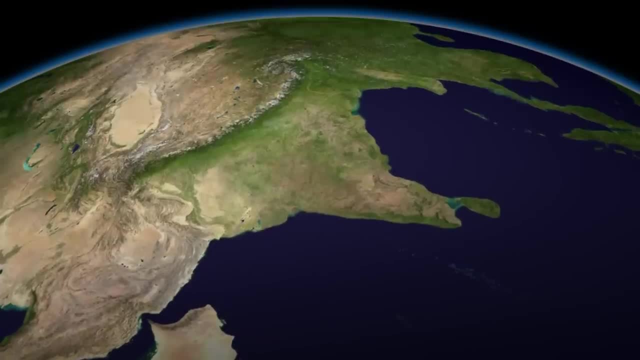 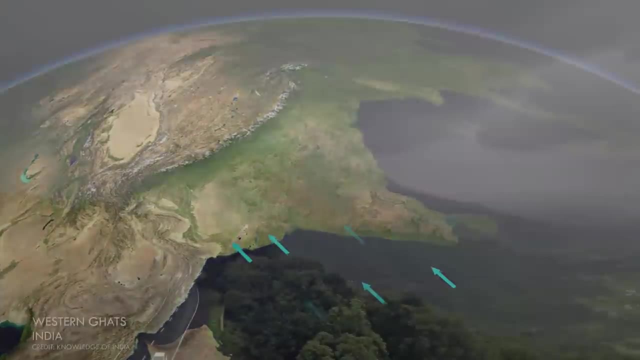 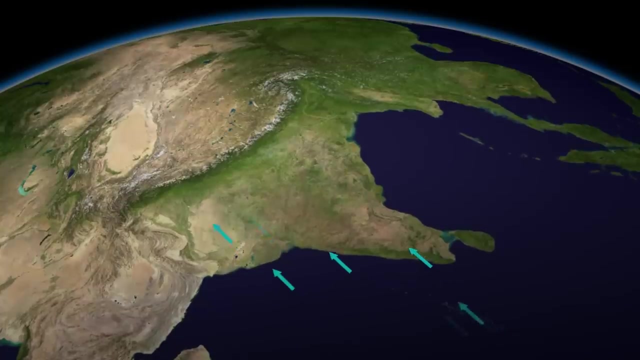 in winter produces a dramatically different result. Now the south-west summer winds blow over the warm Arabian Sea throughout the summer months, bringing in storm after storm that lashes the western coast of India, from Kerala in the south to Gujarat in the north. All along this coast sits one edge of the Deccan Plateau, and these moist winds are 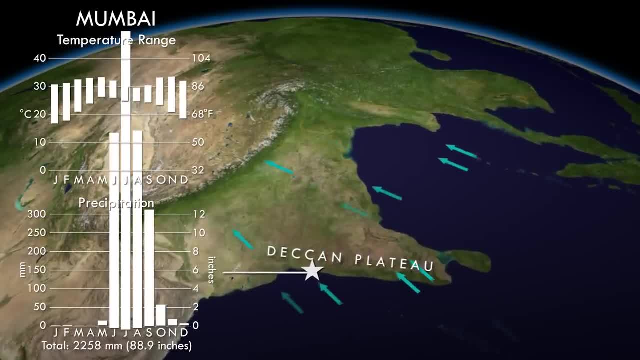 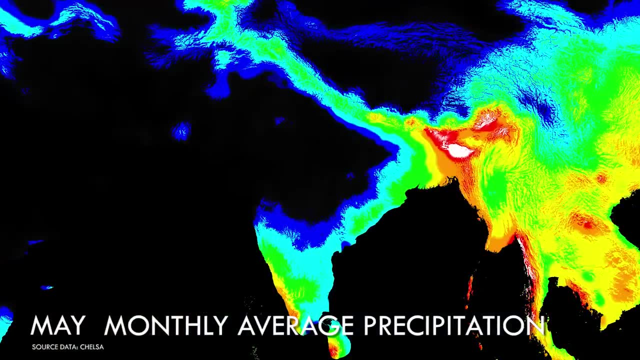 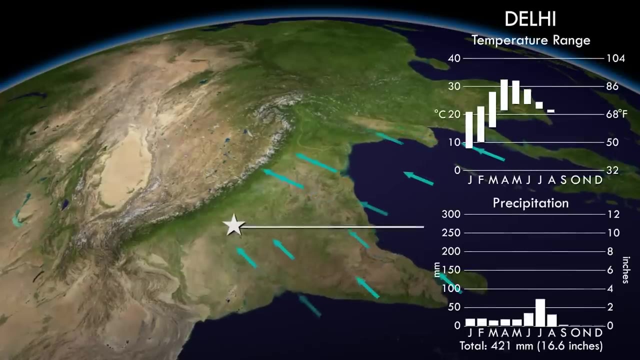 pushed upward and cooled, releasing their moisture in spectacular fashion. as this graph of Mumbai shows, The monsoon progresses across the Indian subcontinent in stages, with the south receiving rains as early as late May and the north as late as mid-July, Protected somewhat by the Deccan. 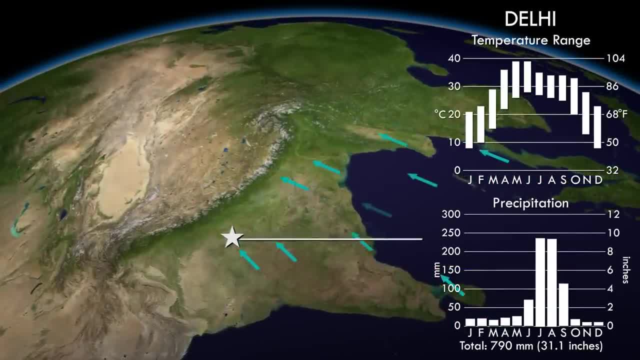 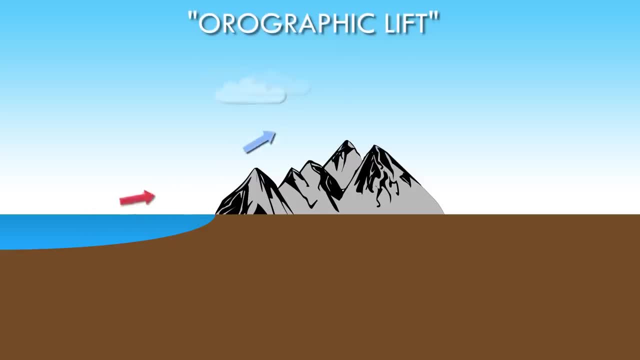 much of the country experiences less severe monsoon rain, But where these strong, moistive, laden winds hit the Himalayas, they are thrust upward in a similar fashion to the west coast and dump almost all their moisture on the windward slopes. And with this mechanism, 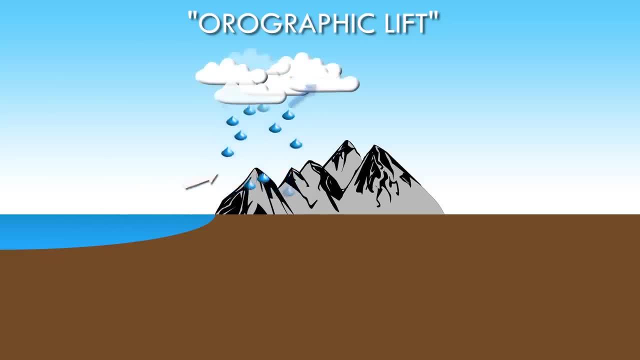 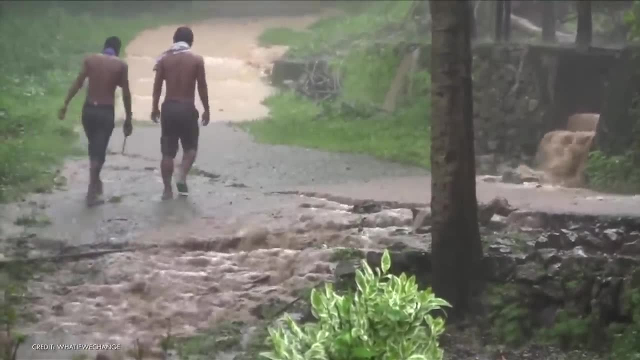 known as orographic lift, we come to a global superlative. The Indian monsoon produces the wettest places in the world. Mohsinram and Cherrapunji, both in the Indian state of Meghalaya, lie in the foothills of 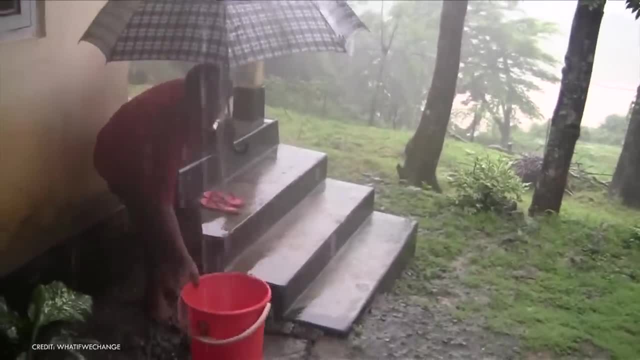 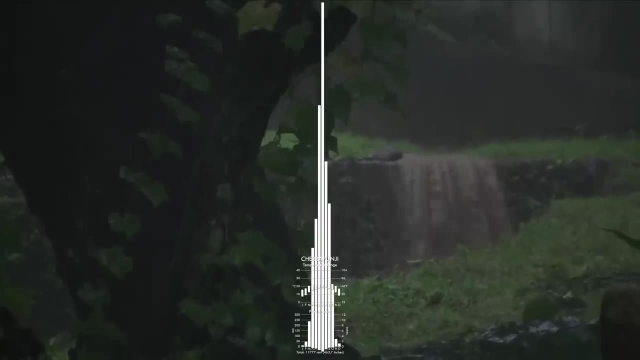 the eastern Himalayas. The Indian monsoon is the most wet in the world and the world's wettest tidal alternates from year to year between these two towns. Here's the graph of Cherrapunji, with the scale kept at the standard used for all my 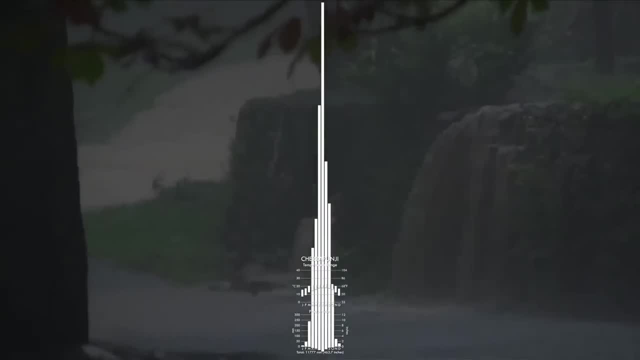 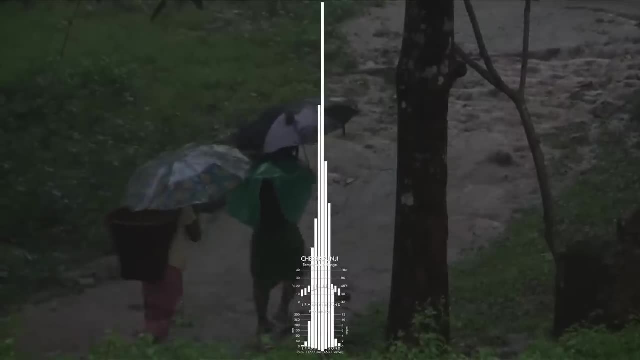 videos just so you can get your head around how much rain actually falls here. In one month alone, at the peak of the summer monsoon, more rain falls here than in an entire year in Singapore, in the heart of the wet tropical rainforest. Three times more rain. 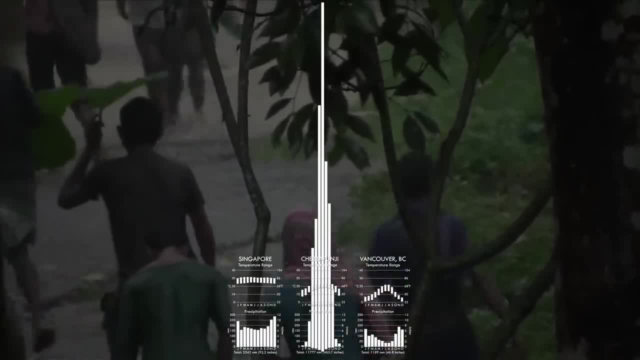 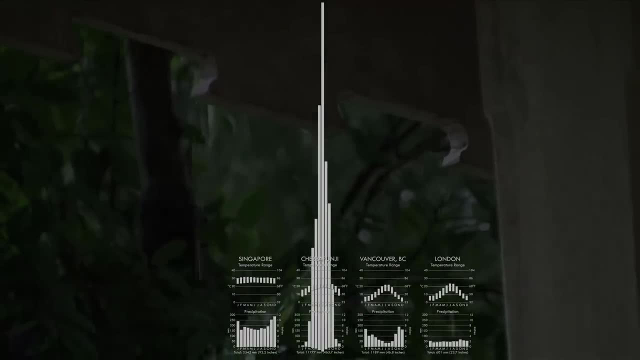 than the annual total in rainy Vancouver And six times more in the winter. This is more than the annual amount in supposedly rainy London. Such is the power of the monsoon. This graph of Lhasa in Tibet shows the effect of the Himalayas Being sheltered from the 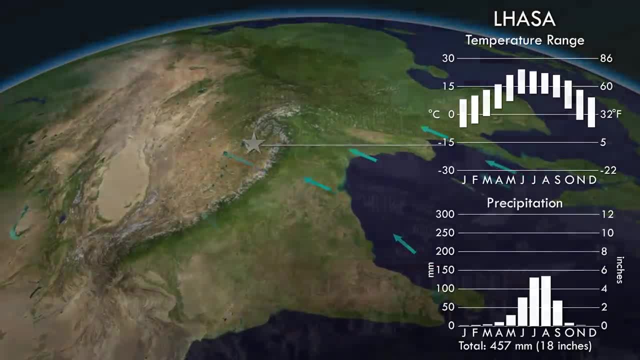 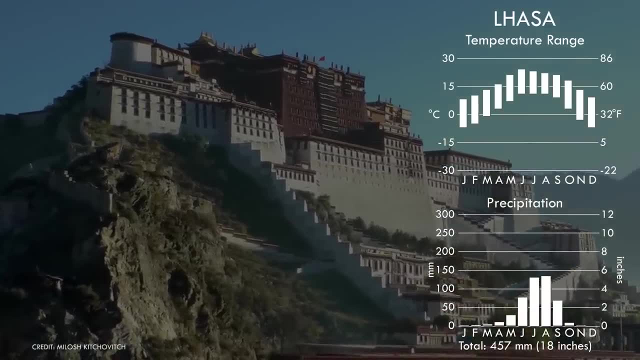 full brunt of the monsoon. behind the highest peaks of those mountains, including Everest, comparatively little rain gets through, although the mark of the monsoon is still clearly visible in the difference between winter and summer. In the Indian winter, the dry northeast wind. 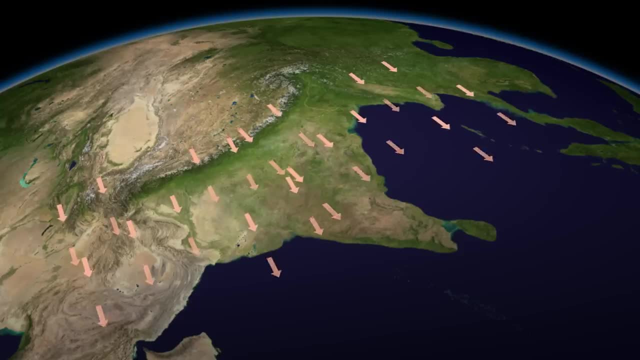 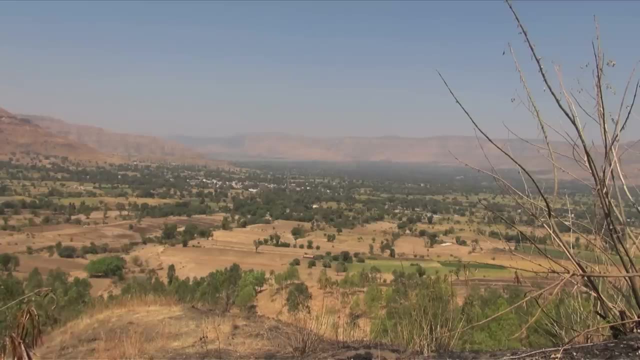 blows from Central Asia out and into the Indian Ocean, Leading to completely dry conditions for months at a time, first with cool temperatures and then very hot temperatures, which leads to the unique three seasons pattern in much of that country: A hot and wet, rainy season. 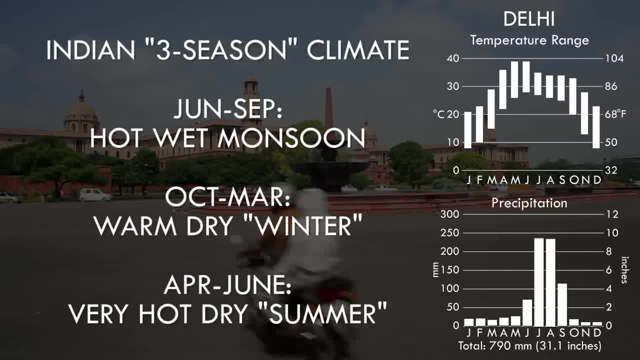 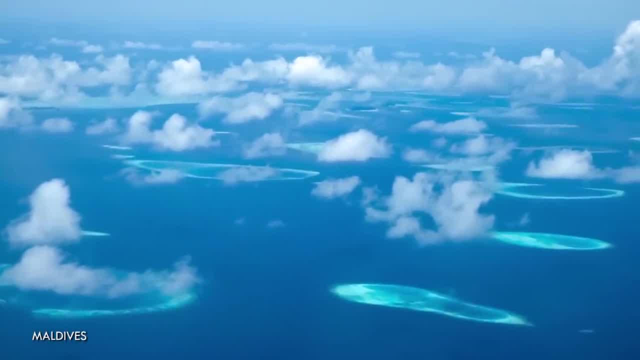 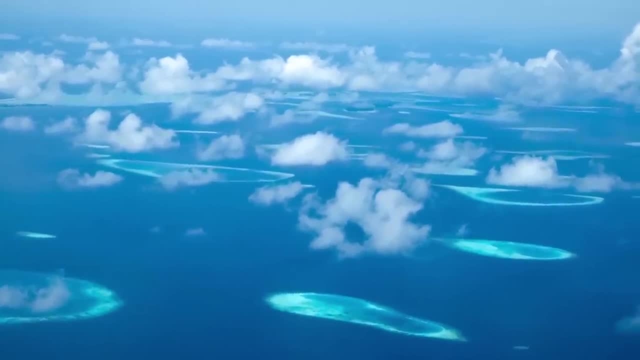 warm and dry winter and then very hot and dry summer. Such is the strength and consistency of the seasonal monsoon winds that they are even able to change the direction of an ocean current. Thanks for watching. A current's direction is primarily determined by the winds blowing over it. 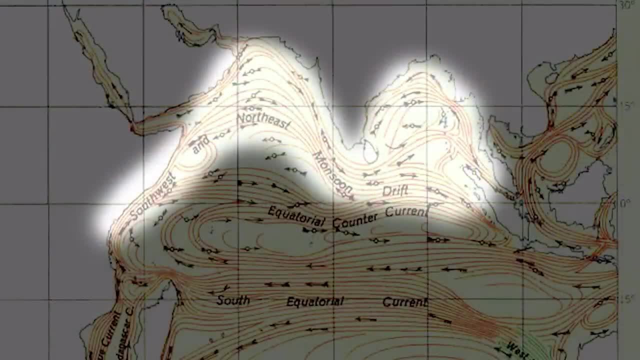 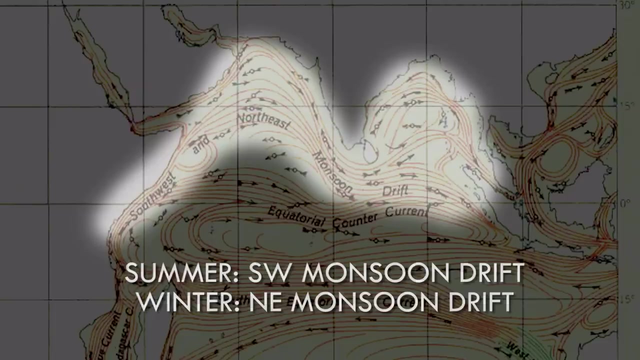 So in summer the current around India flows east, from Arabia to Myanmar, and in winter it flows west. So the name of this current alternates between the South West Monsoon Drift and the North East Monsoon Drift. This is the only major ocean current where such a reversal occurs every year. 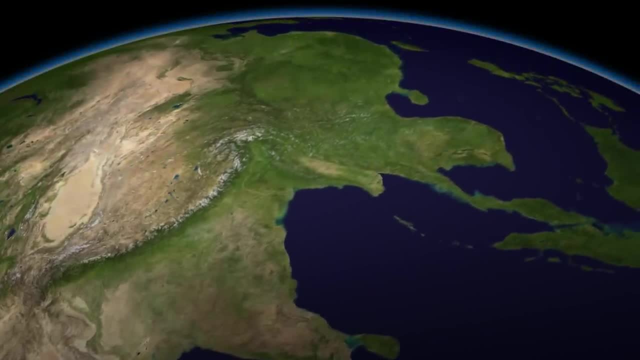 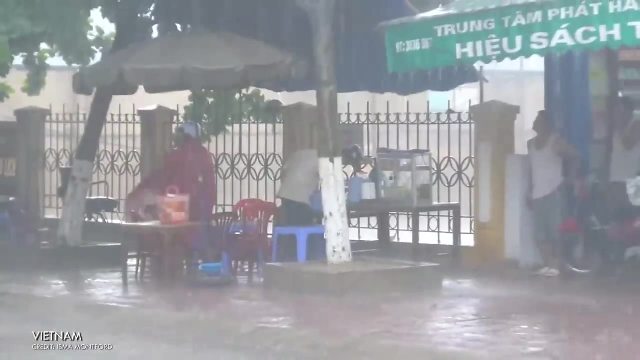 Continuing further east and we pass over South East Asia. This area does feel the influence of the monsoon, but it is within the normal latitudes where tropical, wet and dry seasons occur, with coppen types, AM and AW, predominating. so it does. 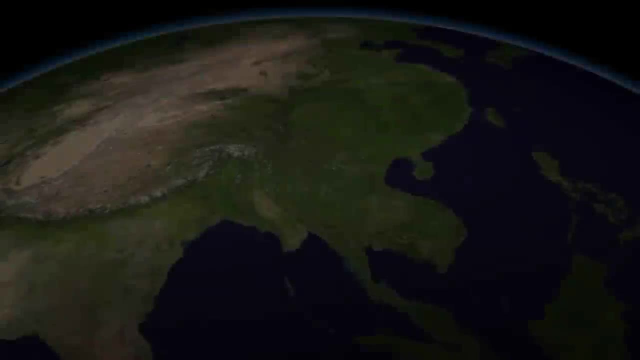 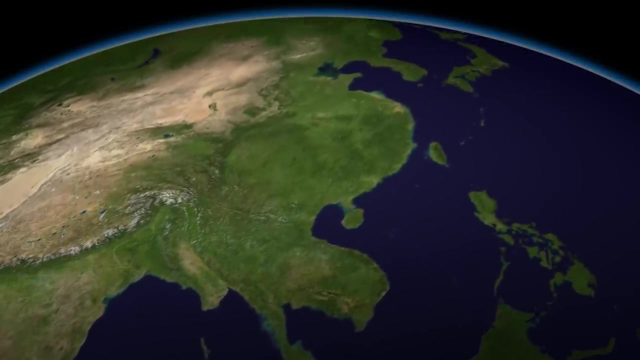 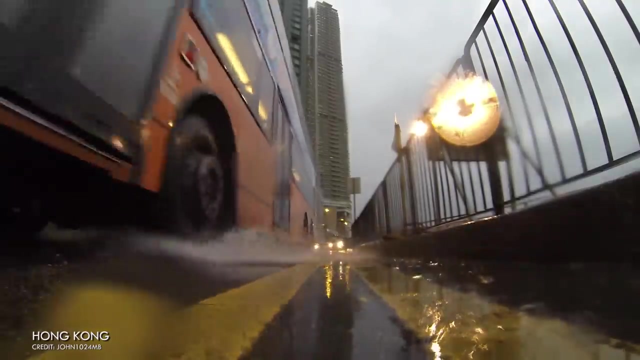 not require special mention in this video. As we continue north and east, however, we enter southern China and the beginning of the East Asian Monsoon. The interplay between continent and ocean now switches to the Pacific, and so we get a different character to that of the Indian – less intense, but spread out over a much. 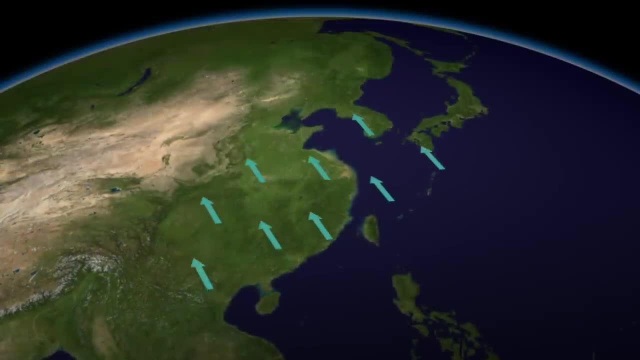 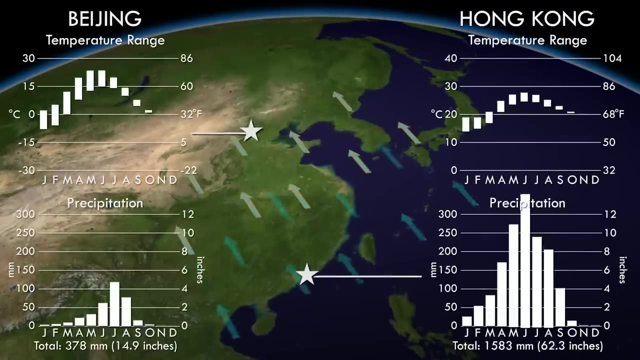 greater area. The monsoon pushes inland hundreds of miles into the heart of China – subtropical in the south, continental in the north – and as one travels further north, the amount of rain and the number of months in which it falls reduces, as the Pacific moisture is. 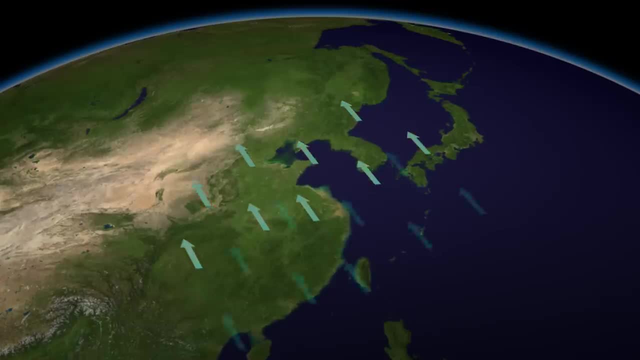 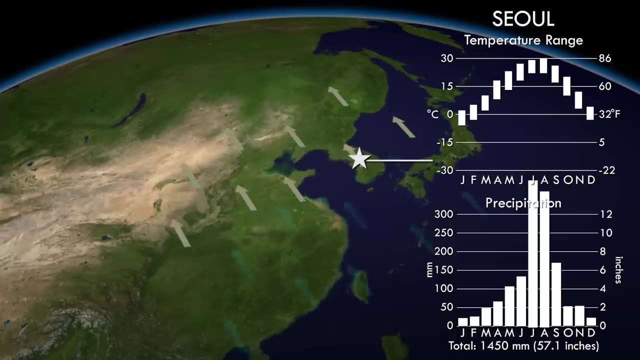 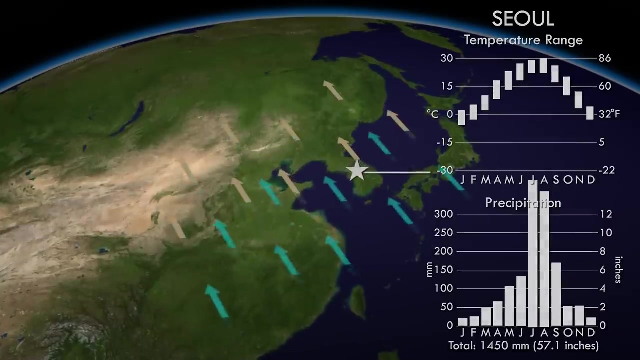 lost over the land, carried by southerly winds. Korea, like northern China, experiences the monsoon as a continental climate, with dry and cold winters blowing in from the Siberian high. but, being on the coast, the monsoon changes, as this graph of Seoul shows. 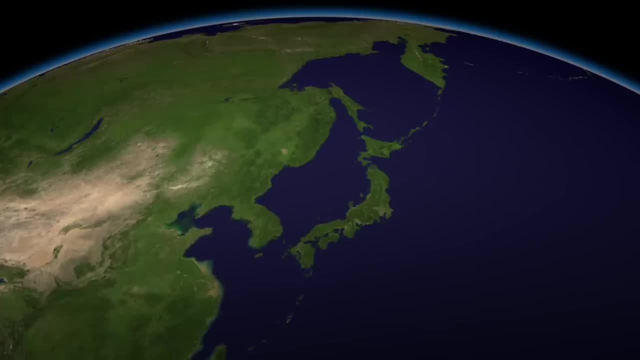 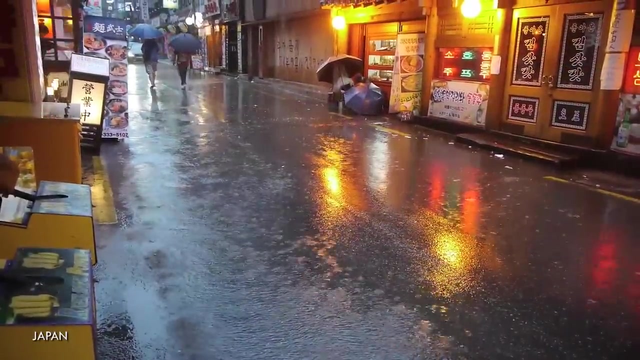 Because Japan is an island archipelago, the change in wind direction produces rain or snow across all seasons, blowing in from the Pacific in summer and in winter across the Sea of Japan that lies between this country and Russia, So one gets a more even distribution of precipitation across the year throughout the islands, although 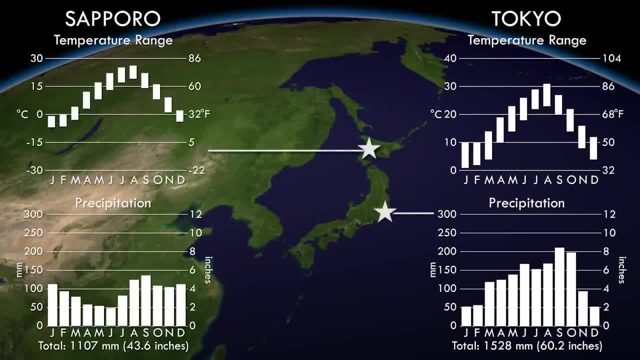 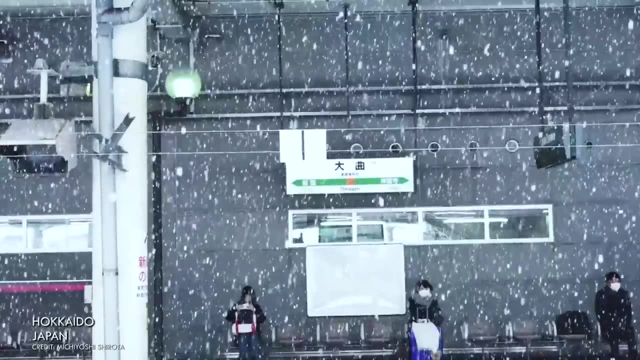 along this mountainous set of islands, the main population centres along the east and southern coasts exist. In fact, Sapporo, the largest city on the northern island of Hokkaido, is the snowiest city in the world, thanks to the winter monsoon winds. 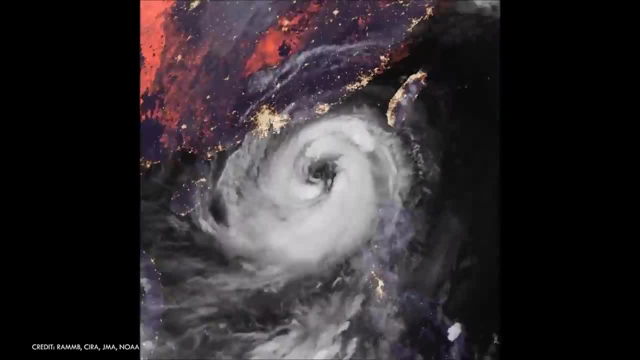 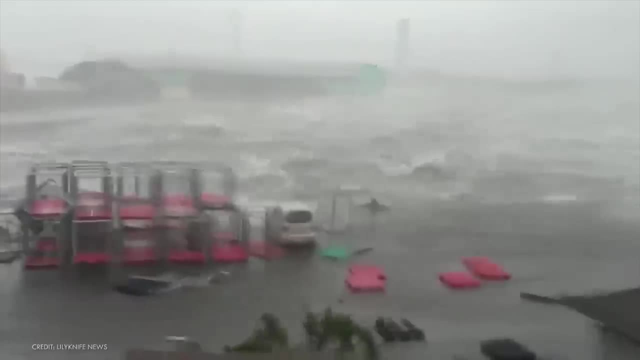 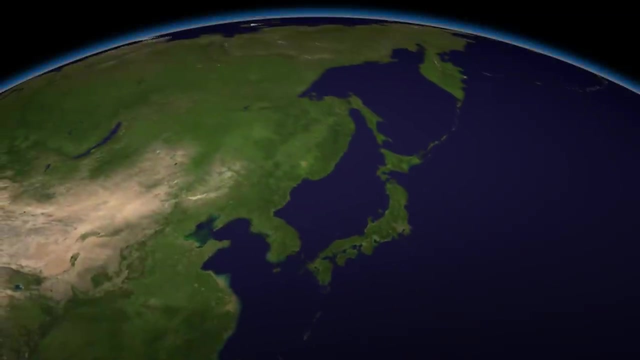 Typhoons in East Asia are another distinction between this part of the monsoon and that of the Indian part. These often ferocious storms account for a considerable proportion of the total rainfall in the season, As they lash cities from Taiwan and Hong Kong in the south, to Japan in the north. 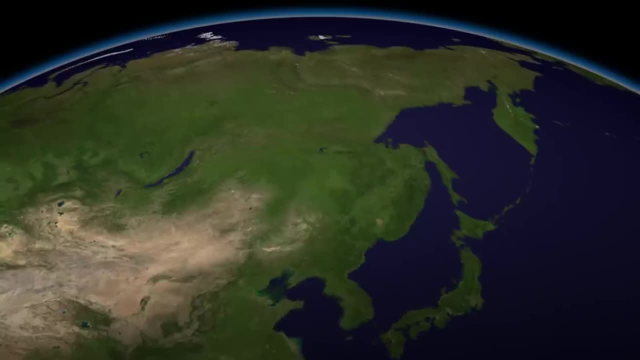 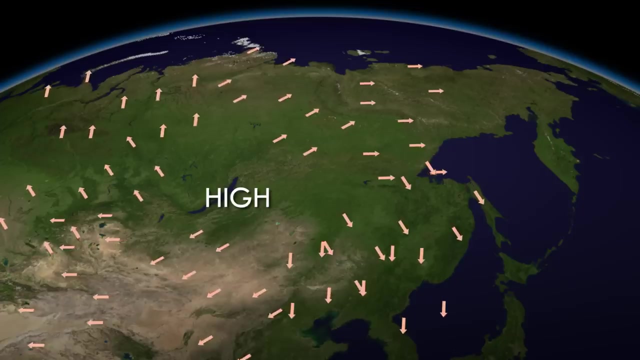 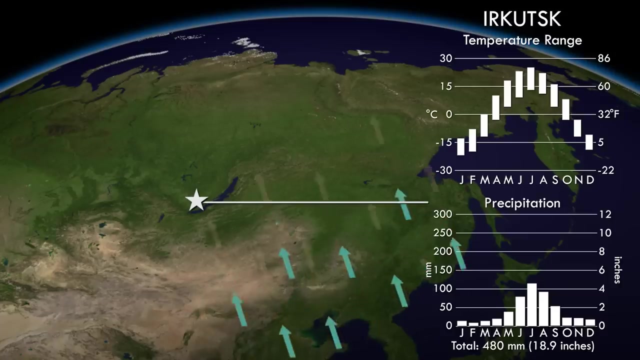 The East Asian monsoon's influence reaches its end in the far north of eastern Siberia, where the winter Siberian high leads to very dry winters. In summer, however, southerly monsoon winds still penetrate this vast area, bringing rain, but by this stage are weakened considerably and the amounts are little compared to those 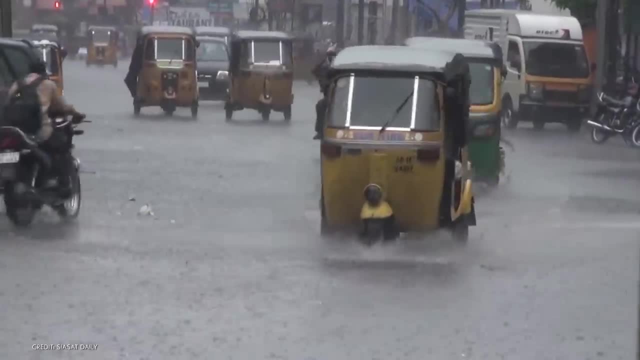 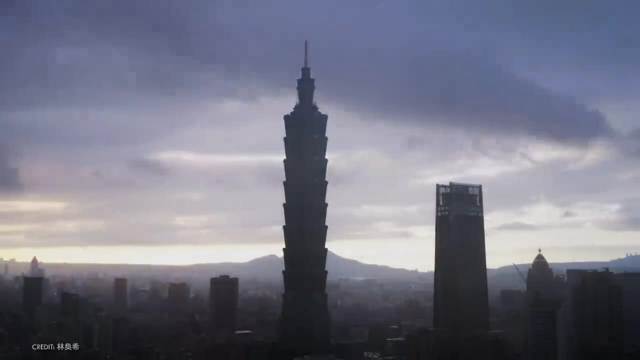 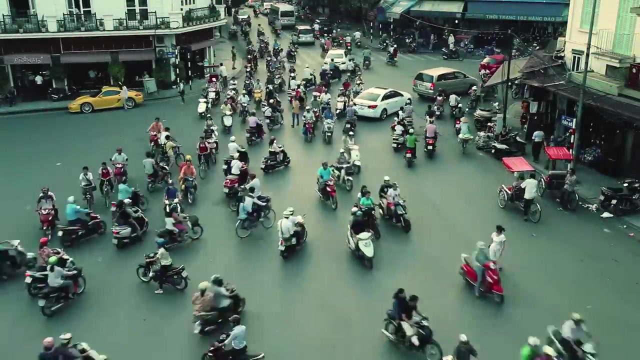 further south. Still, it is a remarkable fact That a singly connected weather system can affect such a large area across so many lines of latitude, from 20 degrees north in India through to 70 degrees north in Siberia. The Asian monsoon varies in intensity from one year to another, affecting both India. 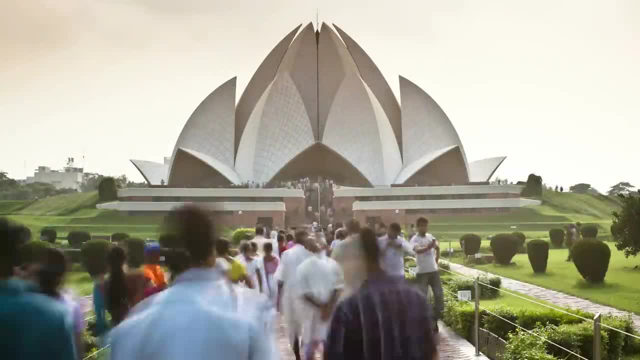 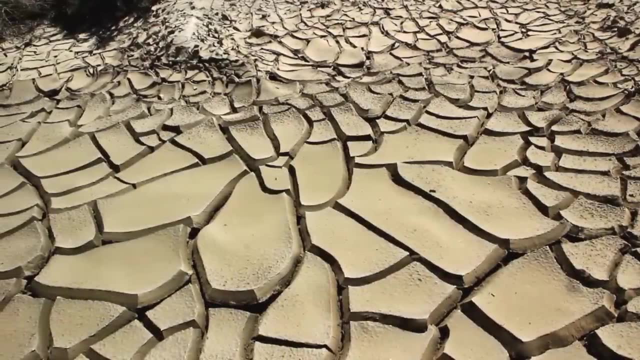 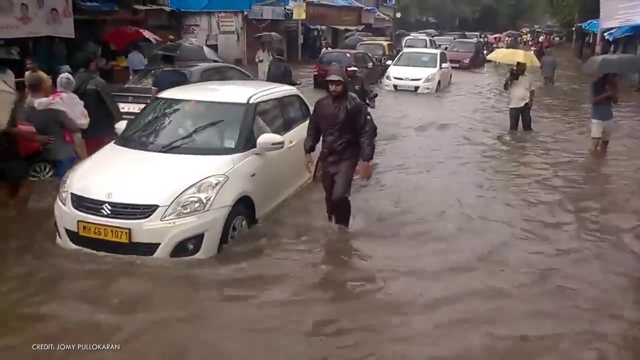 and China. so these average rainfall graphs, as always, can be deceptive in hiding the true pattern of annual variability. Too little rain and effective drought can occur, Since the rest of the year in many places is very dry. already Too much rain and flooding occurs across large areas, in addition to landslides along 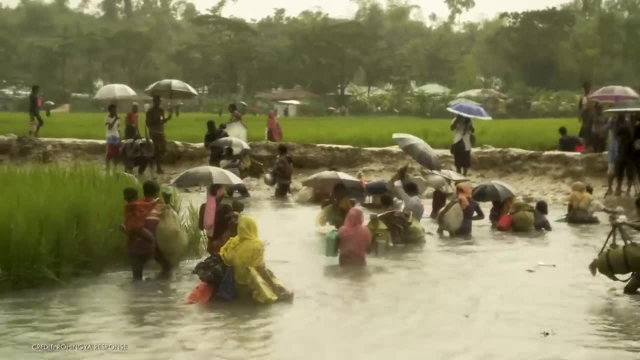 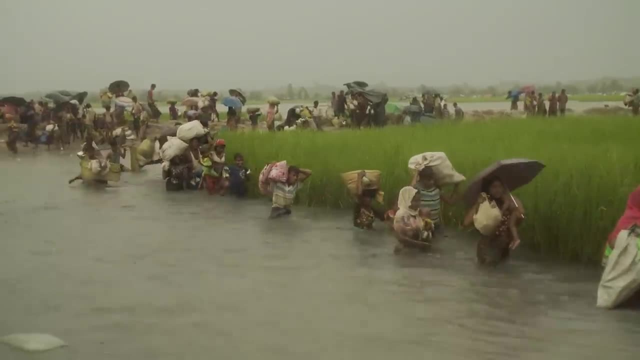 the southern and eastern edges of the Himalayas. Too little and too much rain can lead to many thousands of deaths. in this way, The monsoon is a taker as well as a bringer of life, And that is the Asian monsoon. 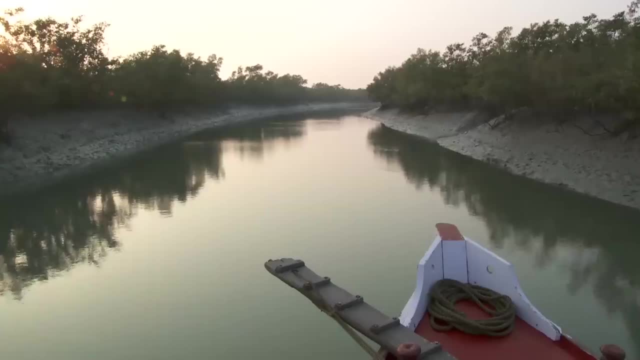 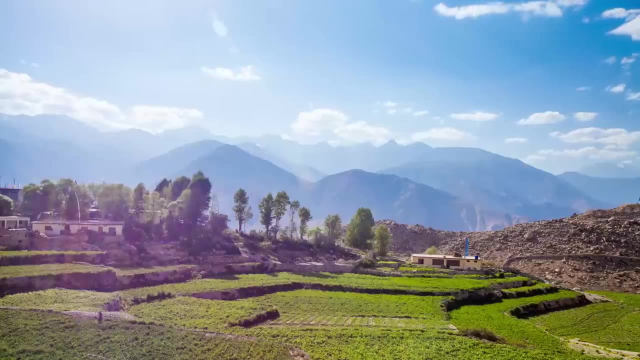 I hope this short video provided you with an understanding of the world of monsoon. I hope you found this video helpful. If you have any questions, please leave a comment below. It is the world's largest and most important weather system. If you live in this region or have visited during the rainy season, then I'd love to 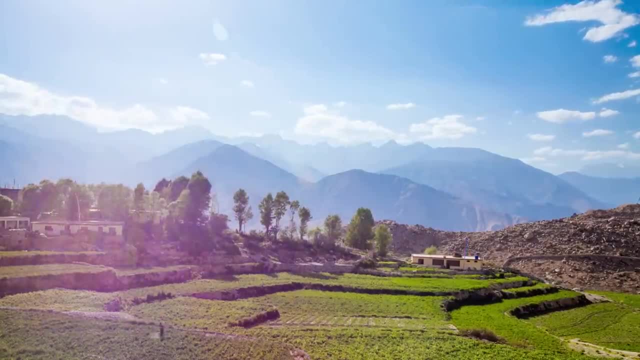 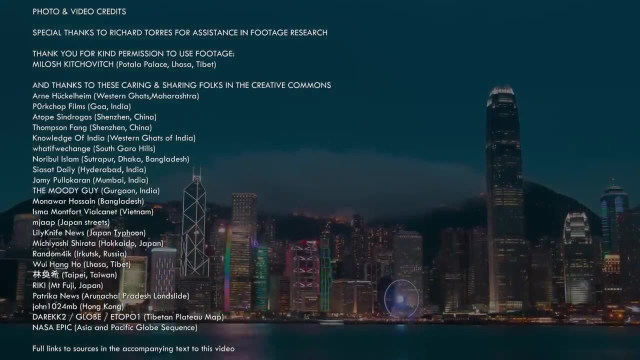 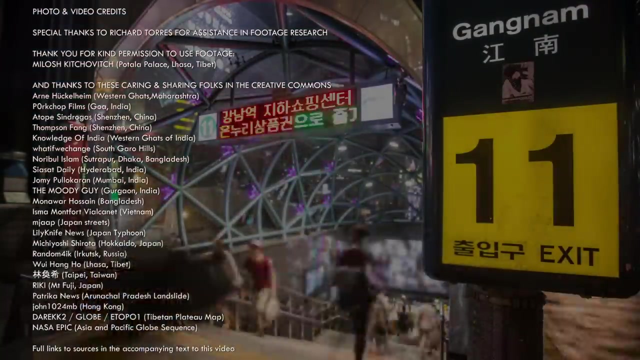 hear of your experience of the monsoon in the comments, As always. if you enjoyed this and other videos of mine, please click the subscribe button so you don't miss future episodes. and don't forget to like and share this video. Thanks again for watching and I'll see you in the next of the Climate Casebooks series. 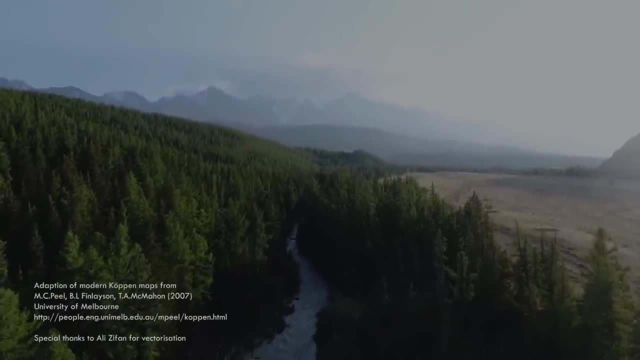 Bye, Bye, Bye, Bye.